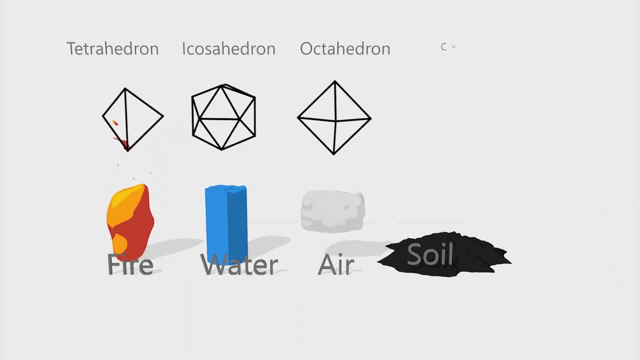 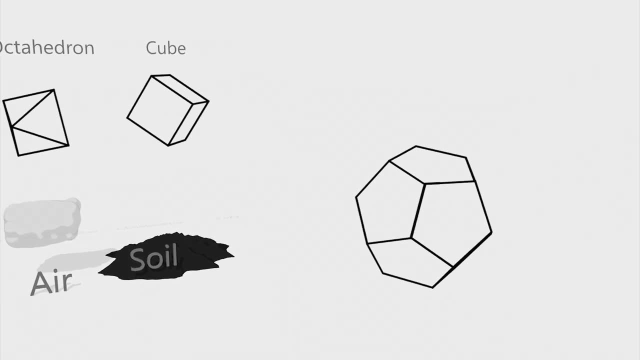 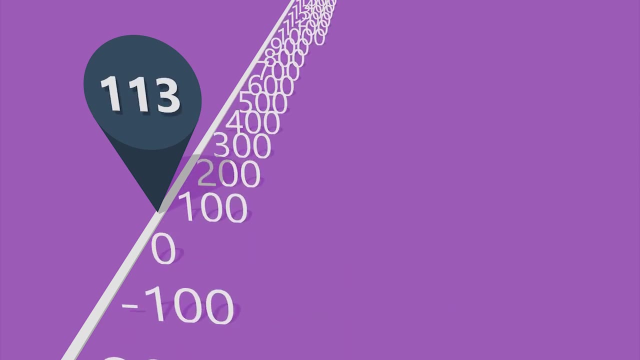 3d geometric figure: the tetrahedron, fire, icosahedron, water, octahedron, air and finally the cube soil, and then something to represent the universe: slash, the ether, the doctahedron. But then nothing happened for atomic physics for quite some time. So we started in 400 BC and it's not until we meet John. 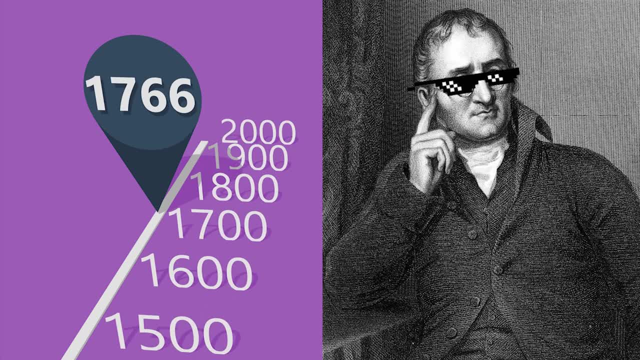 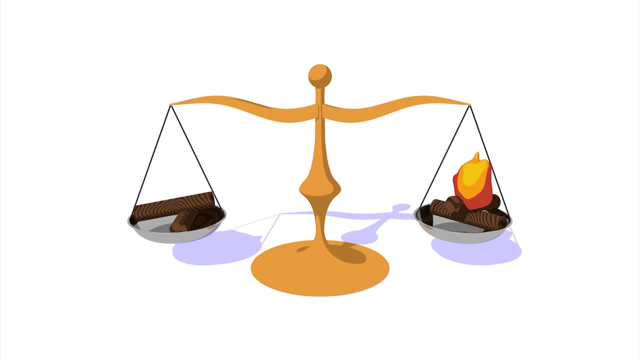 Dalton in 1766. something happens again. Well, in chemistry there was some development at least. It was found that if you have a system, say some wood, of course if you set fire to the wood it will lose mass. but it was found that if you isolate the system no mass was lost. Also, it was found 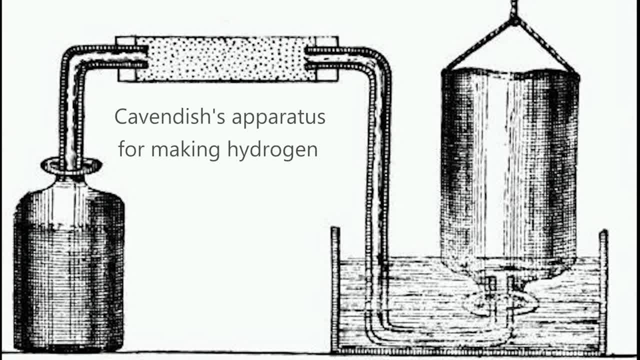 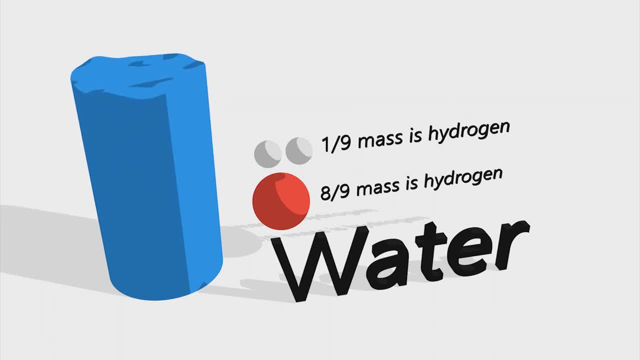 that some compounds couldn't be broken down further, like hydrogen and oxygen. It was also known at the time. if you have a chemical compound, say water, it will always contain the same ratio of mass of the different elements. Adding more or creating more won't change that ratio. So 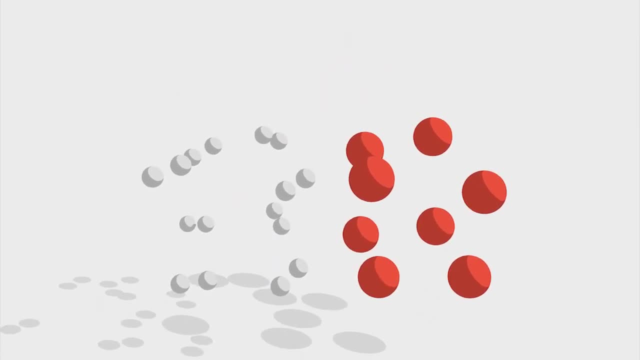 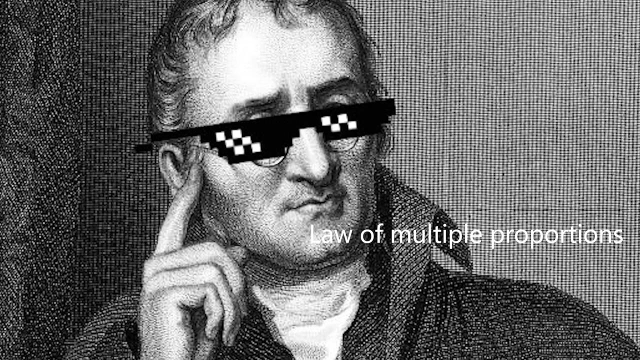 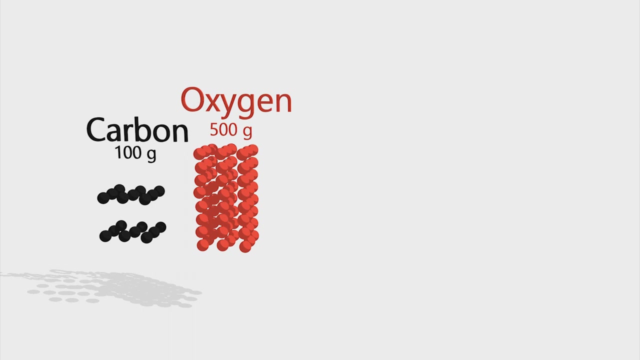 it always contains this much hydrogen and this much oxygen. That's kind of obvious now where I use the modern picture of molecules. John Dalton created a new law called the law of multiple proportions. It states if you have two elements that can combine into multiple compounds- say 100 gram of carbon and 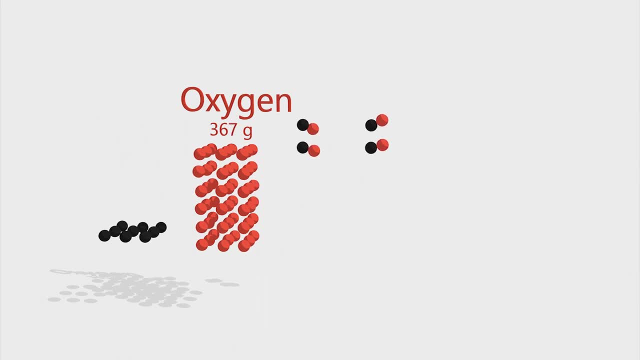 500 gram of oxygen. it can combine into carbon monoxide. Then it will take 133 grams of oxygen in the process. It can also combine into carbon dioxide, taking 266 grams of oxygen in the process. Now, finally, here is what the law states. If I take the, 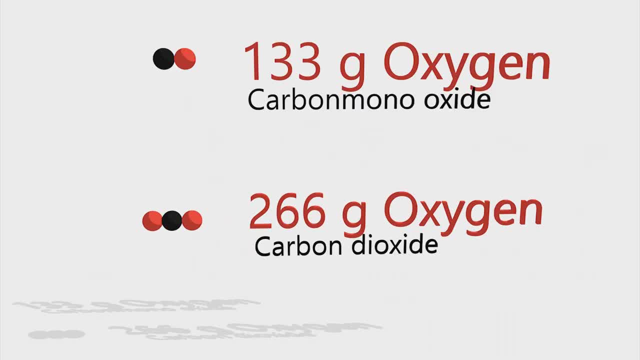 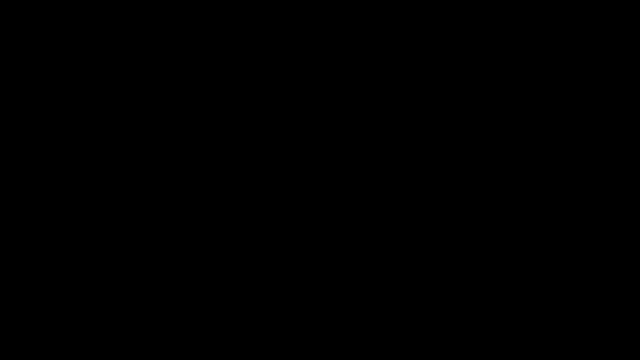 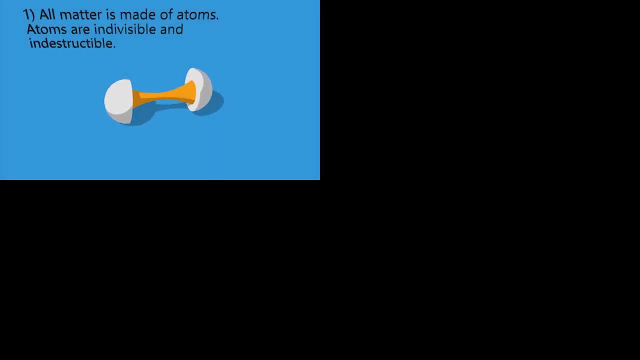 second element, in our case oxygen, and I divide the masses used in different processes, I will always get a small integer value From all these laws. he developed and hypothesized the following atomic rules: One: All matter is made of atoms. Atoms are indivisible and indestructible. Two: All atoms of a given 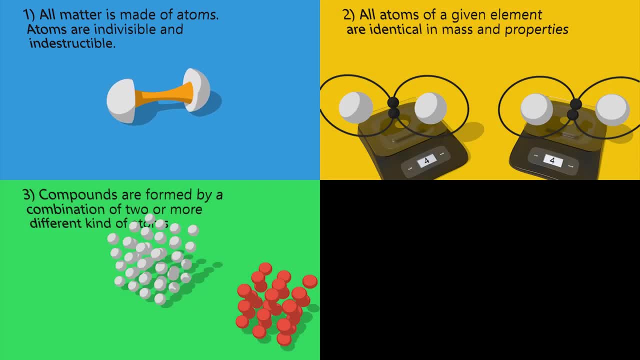 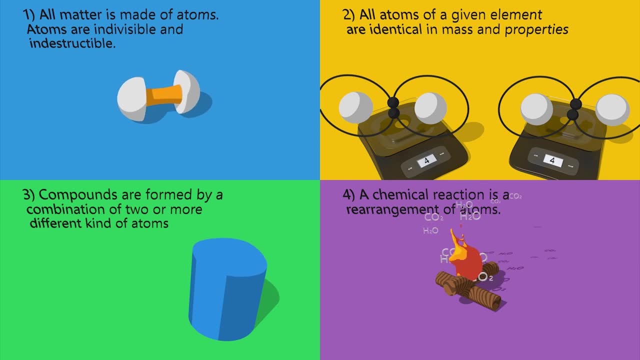 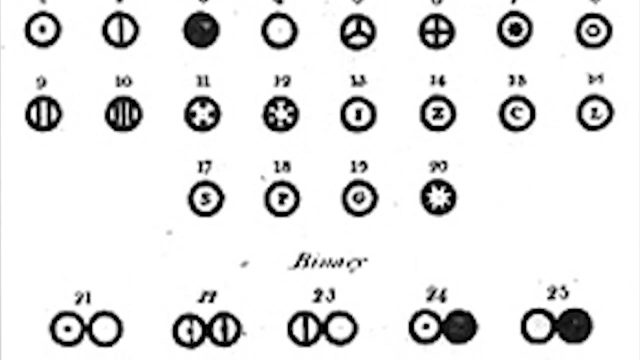 element are identical in mass. Three Compounds are formed by a combination of two or more different kinds of atoms. Four: A chemical reaction is a rearrangement of atoms. Everything wasn't perfect, but it is the first real try of an atomic theory. And here we see some of his sketches. but he 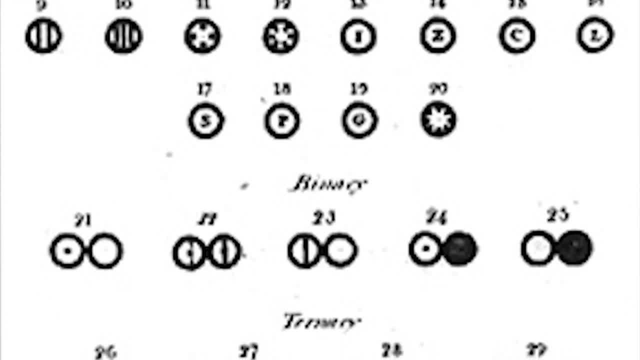 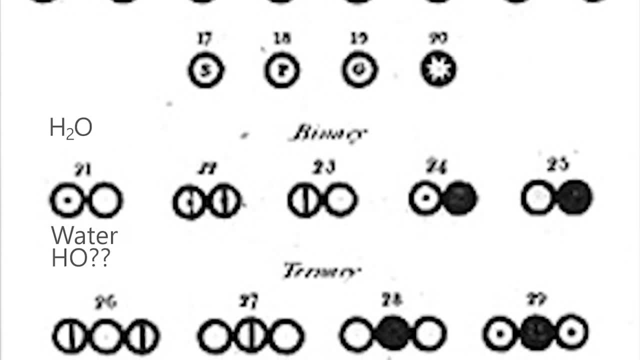 thought that the simplest compound between two elements is always the same, So he thought that the first one is always one atom each, Which is obviously not correct. Here you can see that he thinks that water was HO and not H2O. Will Josef Gay-Lucas and Alexander von Humboldt fix that So? 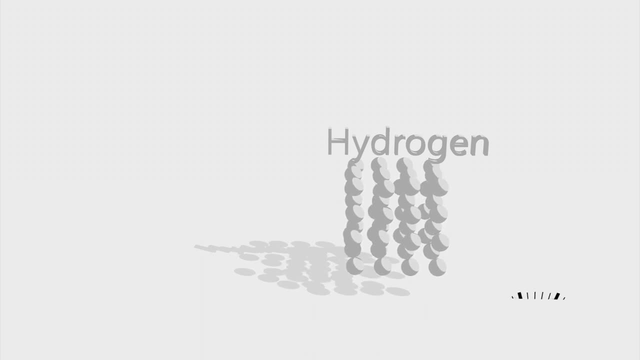 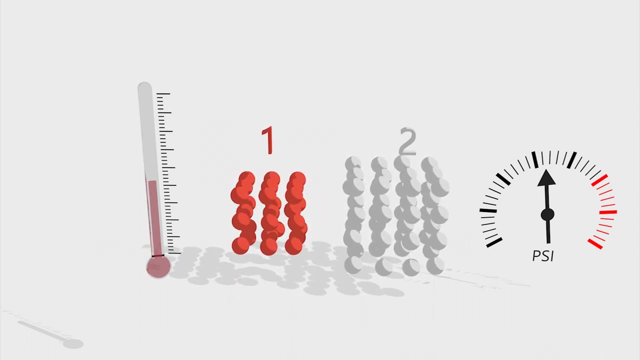 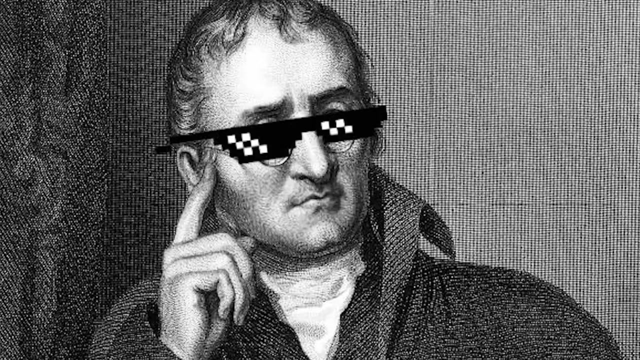 they saw that hydrogen will always, at the same pressure and temperature, occupy twice as much value as oxygen if it had to completely recombine into water, Suggesting that water is two part hydrogen and one part oxygen. So that fixed John Deltz's problem. 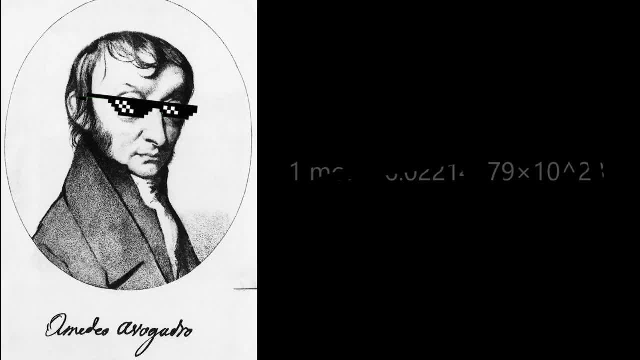 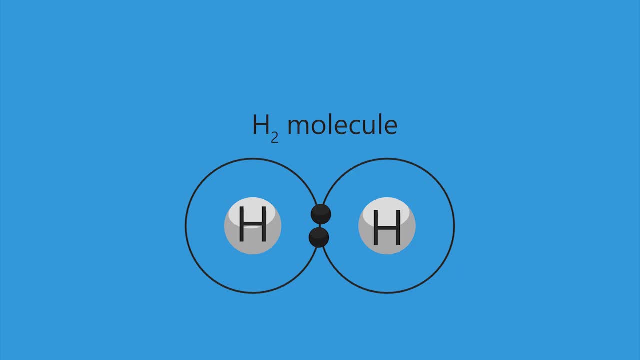 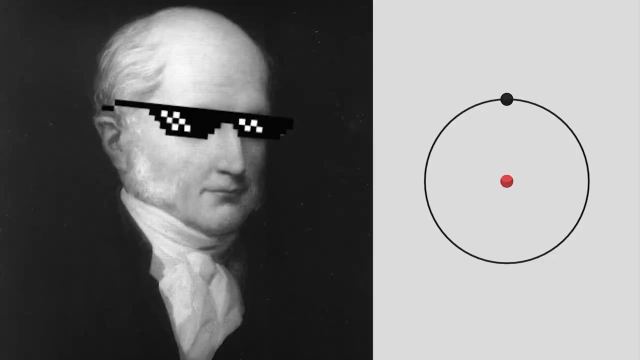 Up comes Amadeo Avogadro, and you know, he of course introduced the mole. He also concluded a molecule consists of one or more atoms, which John Deltz didn't know. And of course he helped develop the gas theory, The ideal gas law. William Prout suggested that everything was made up from. 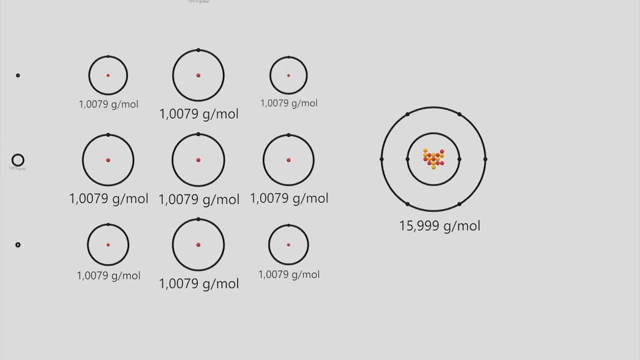 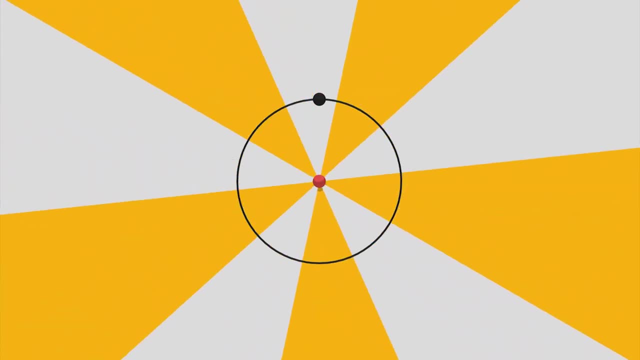 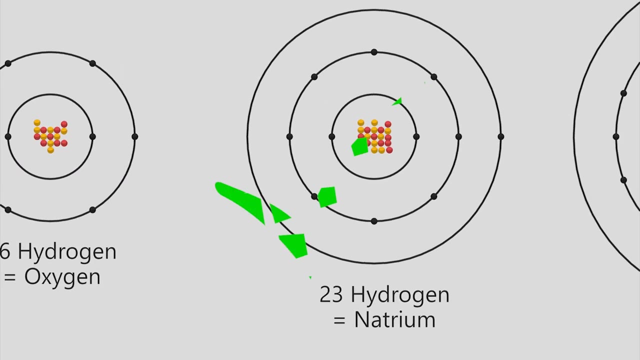 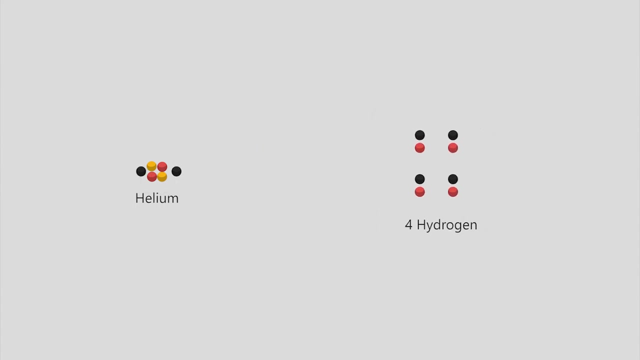 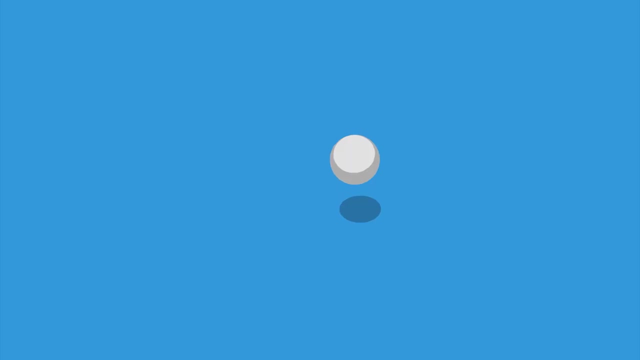 hydrogen. He saw that, for example, oxygen weighed almost the same as 16 hydrogen. So he thought that hydrogen was the true fundamental objects and he called hydrogen hydrogen. So he thought that hydrogen was the true fundamental objects and he called hydrogen a protyl. Almost all of the known substances at the time followed this rule That the weight was always n times hydrogen. It was, however, not correct, because the proton and the neutron does not weight the same and the electrons did not match up at all, But they are not that heavy. So when they found an element that didn't follow this rule, they thought maybe there is something fundamental about hydrogen instead And started looking for what hydrogen was made up of. 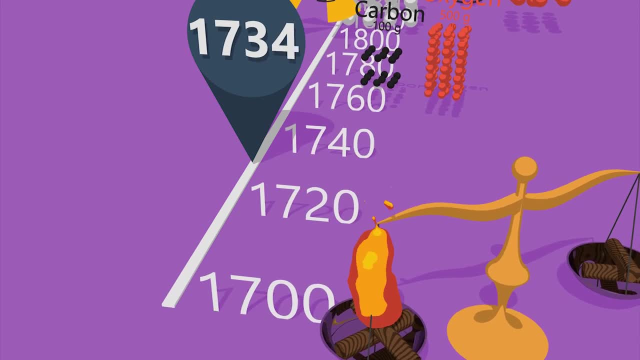 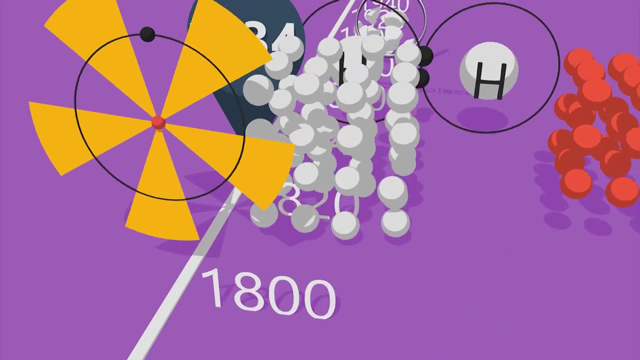 So many things. Let's recap really quickly. We learned about the conservation of mass, Jay Dalton's various laws, John Dalton's law of multiple proportions, Some gas relations, the protyl- what a molecule is, and finally, Prout's hydrogen weight. 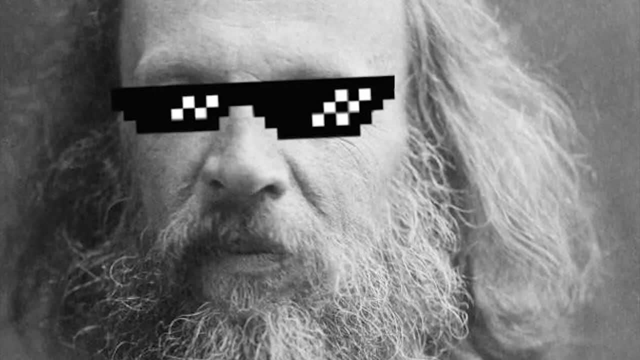 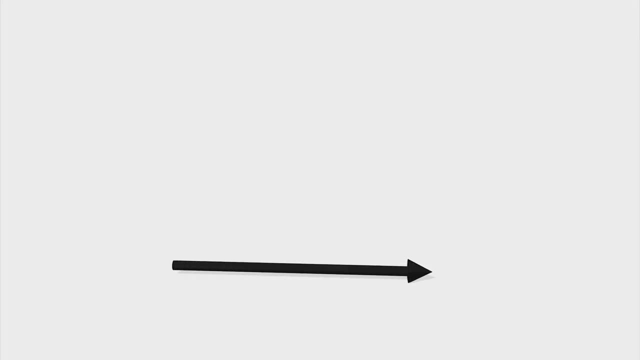 hypothesis. I want to go through one more guy, Dmitri Mendele, a chemist, decided to play a round of solitaire with atoms. He arranged the known atoms in rows by chemical properties and in columns by atomic weights. He predicted unknown elements because when he arranged the known 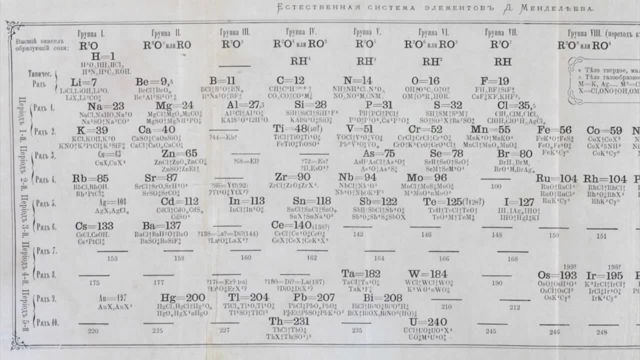 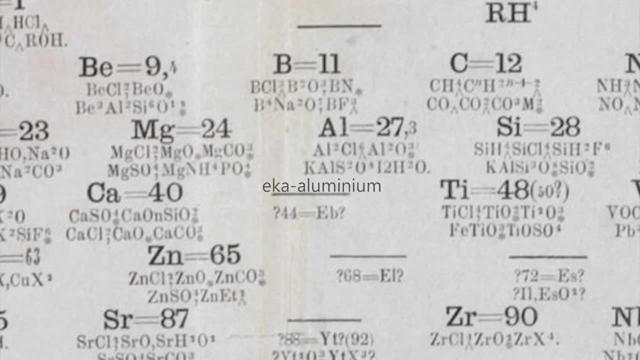 elements. there was holes in his system. For example, here is his early table. He predicted an element should exist right under aluminium and called it Eka-aluminium. It was later found within his life span. there is indeed an element, and we called it Gallium. The model wasn't perfect.